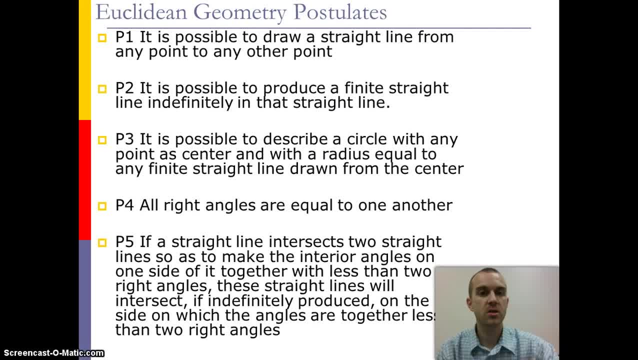 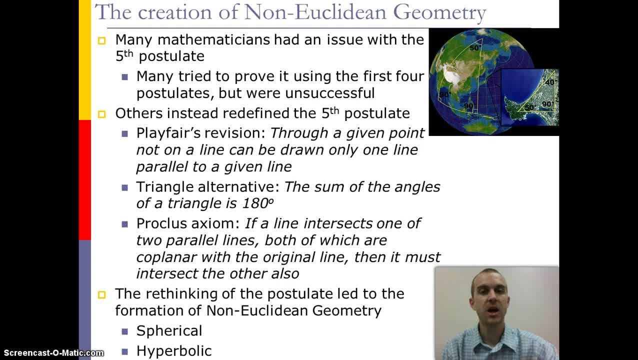 In this video we'll explore non-Euclidean geometry. Now, Euclidean geometry started with five postulates, but it was the fifth one that gave everyone so much problems, to the point where people were trying to prove the fifth based on the four first postulates, and it's been revised along the way to try to make it make more sense to people. 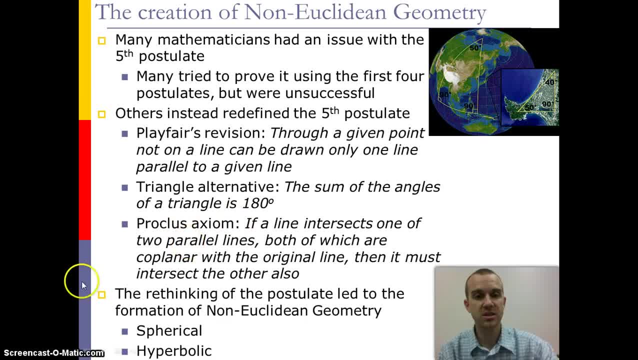 The revision that we often teach our students is Playfair's revision that through a given point, not on a line, can only be drawn one line parallel to a given line. But there have been other ways people have viewed it, for example the Triangle Alternative, Proclus, Saxion. and it's because people continue to try to rethink the fifth postulate that we see the creation of both spherical and hyperbolic geometry. 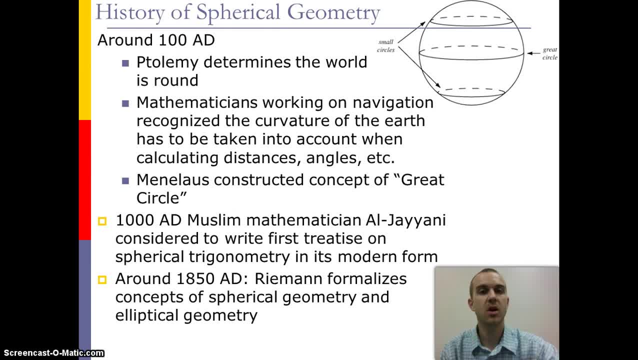 Now spherical geometry started with the concepts from the Greeks. Ptolemy determined that the world was round around 100 AD, and they started to use that concept in the idea of how they calculated their distances and angles when dealing with situations on Earth. 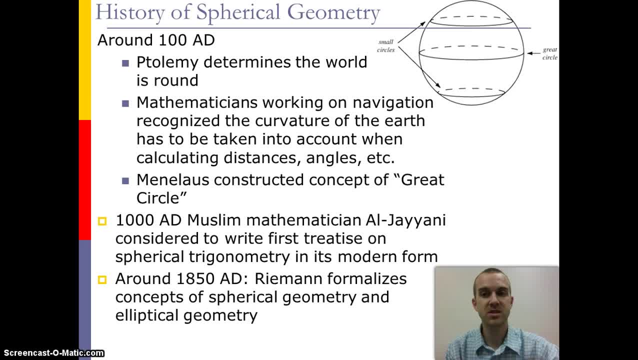 Menelaus then came up with the idea of the Great Circle being what would be considered a line on a sphere, And then from there, a lot of the major, significant work then came from the Arab nation- mathematicians, For example. 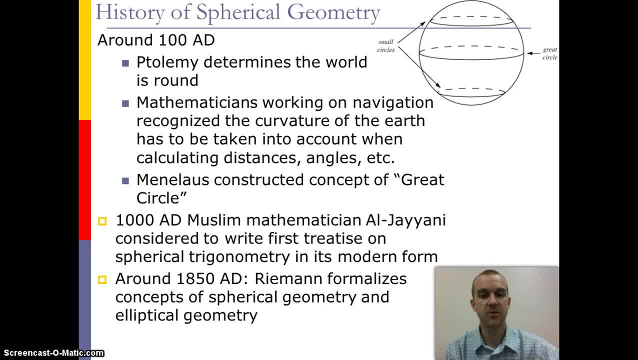 Alajana considered to write the first treatise on spherical geometry in its modern form, and then it's been continued to be improved upon from the Arabian mathematicians, And around 1850, Riemann formalized the concept of spherical geometry as well as elliptical geometry. 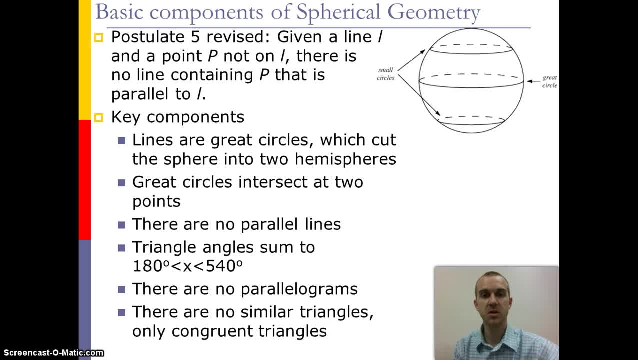 Now here are some of the basic components to understand about spherical geometry. The way that the fifth postulate's revised is that, given a line L and a point P, not on L- there is no line containing P that is parallel to L. 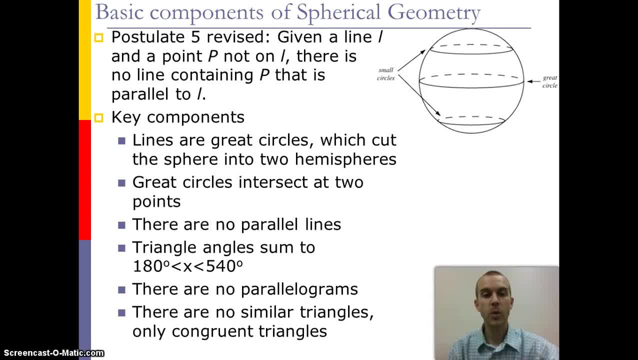 And this is the fact that in spherical geometry we consider only great circles to be lines. So because lines have to split the sphere in half And the only way that's possible is if two of the great circles intersect, So there's no way to make a parallel line in spherical geometry. 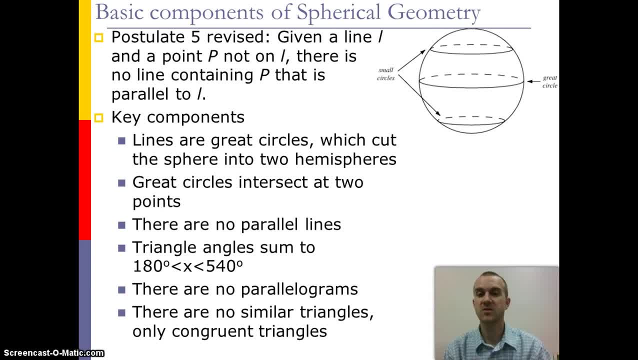 Triangles are actually going to measure from 180 degrees to 540 degrees And because there's no parallel lines, there can be no parallelograms And there are no similar triangles. If you have a triangle, it is congruent but not similar. 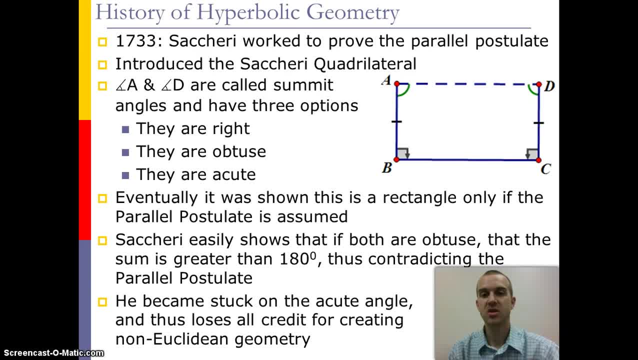 Now hyperbolic geometry took on didn't start to be discovered until the 1700s, when Ciceri worked with the idea of trying to prove the parallel postulate. He created the Ciceri Quadrilateral in which we're trying to. 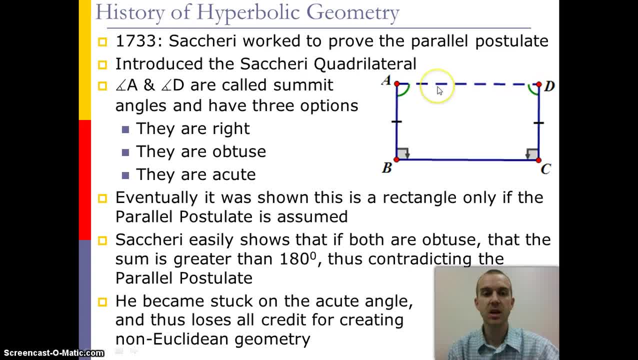 where you look at points A and D or angles A and D and call them summit angles, And we recognize that they have to have one of three options: They're either right, obtuse or acute. If it's right, we have a rectangle. 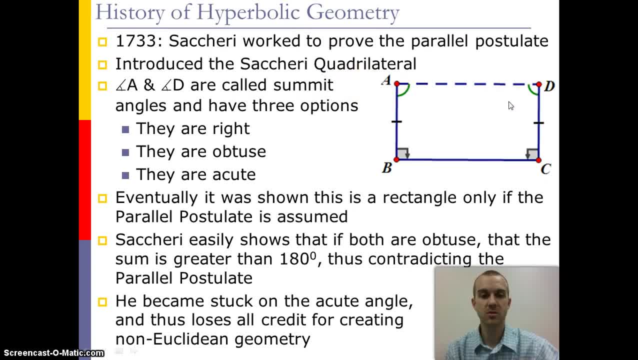 But then he started to look at, well, what happens if these angles are obtuse or acute, And what he noticed was that, if they are both obtuse, that the sum is greater than 180 degrees, Which contradicts the parallel postulate. 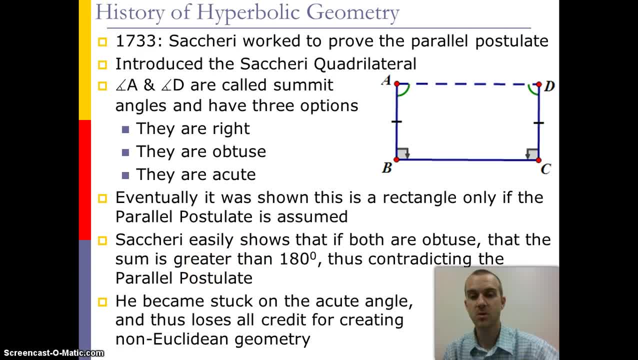 But then he tried to continue to work on this quadrilateral with the acute situation And because he got lost doing that, he never completed his work And then ends up losing all the credit he could have been known for for non-Euclidean geometry. 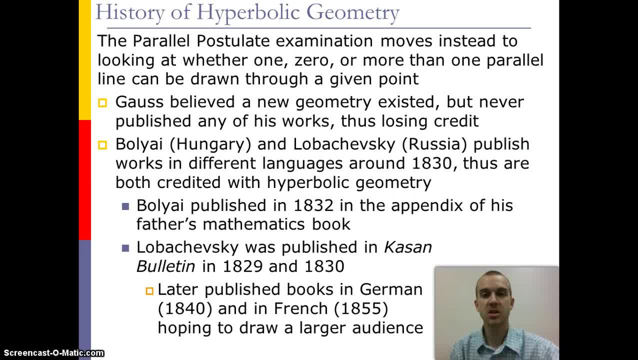 From there the parallel postulate moved to instead of looking at whether one zero or more than parallel lines can be drawn through a given point. Gauss did a lot of work with this, And he thought that there was some other form of geometry, but just never published anything. 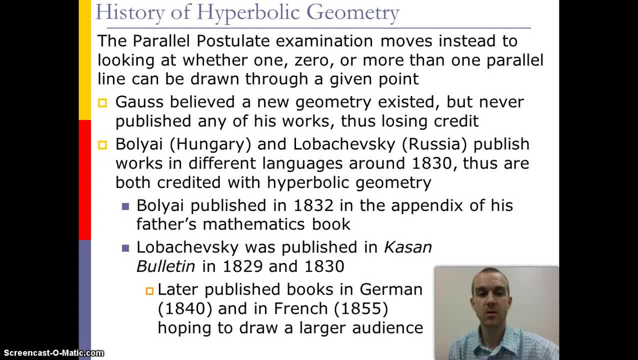 So he didn't get credit for it, And the two men that end up getting credit are Bolya and Lobachevsky. And Gauss even wrote to Bolya's father commending his son for the work that he'd done. 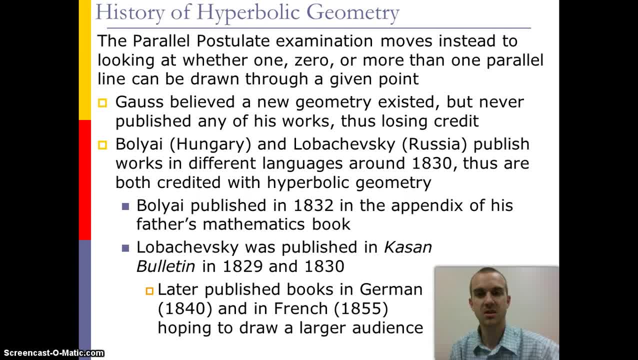 saying that he found the concepts that just had continued to elude him, And Bolya then accused Gauss of trying to plagiarize and steal his work. And the reason we give both of these men credit is because they published in the same year in different languages.